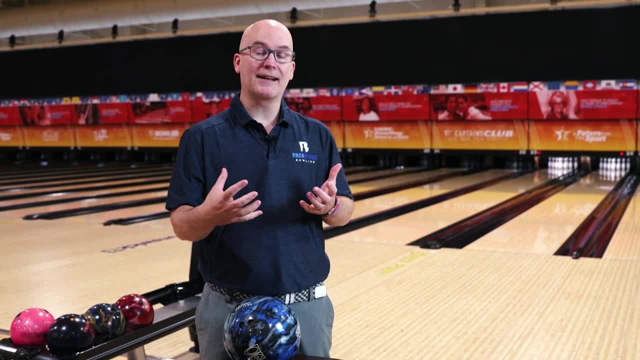 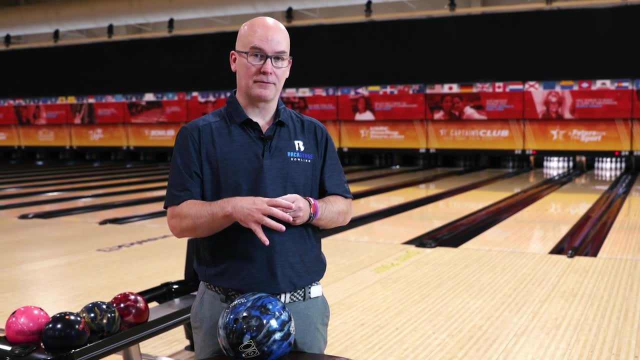 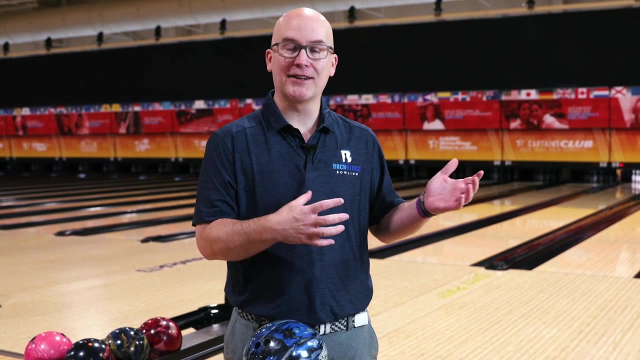 doing things properly on the lanes. So what I want to do is diagnose and give you guys at home quick tips that can help you diagnose whether or not your ball fits you properly. So first, hole size. You know a lot of people they're a little bit worried that they're going to go down the lane. 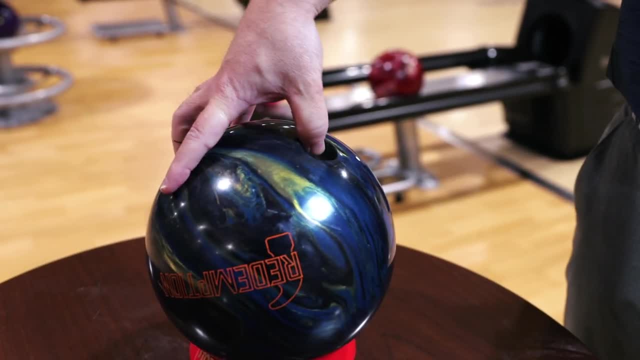 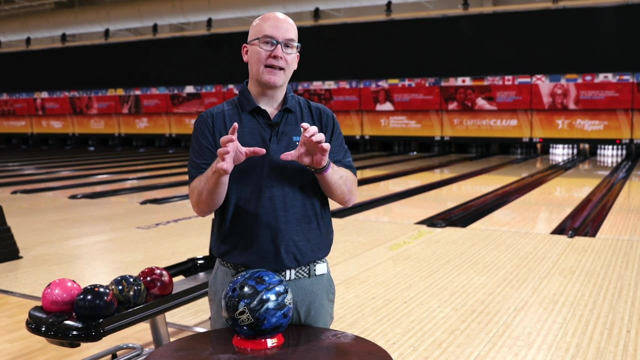 with a bowling ball. So they end up having the hole size be way too loose and they end up having to squeeze it a lot to hang on to it. So we want to make sure that the thumb hole is tight, but not so tight that we're going to go down the lane. So that's something that, as you get greater and 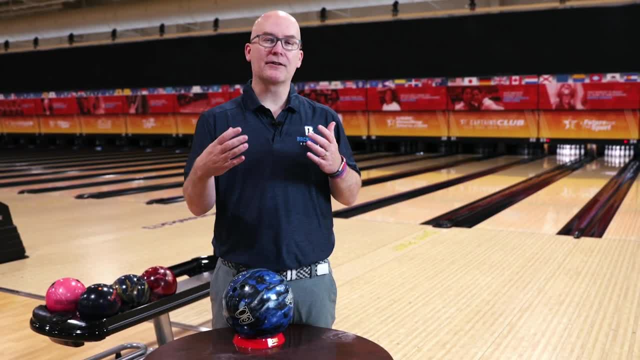 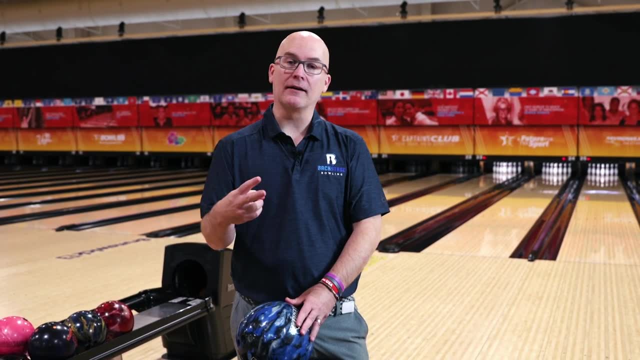 greater skill levels and you become more advanced as a player, you should be able to start to fine tune your feel and touch to get that hole size nice and snug. So the second thing we're going to do is we're going to go down the lane Once again. that's the distance apart between your 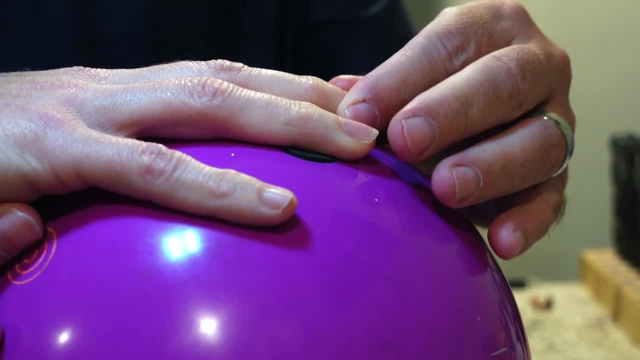 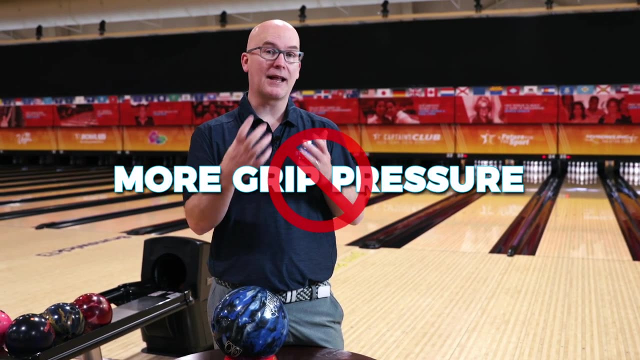 finger holes and your thumb hole. If that gets to be too stretched or too short, you have to use more grip pressure to hang on to it. Remember this is kind of the golden rule. More grip pressure in bowling is bad. We want to be as relaxed as possible so that our swing can stay nice and loose. 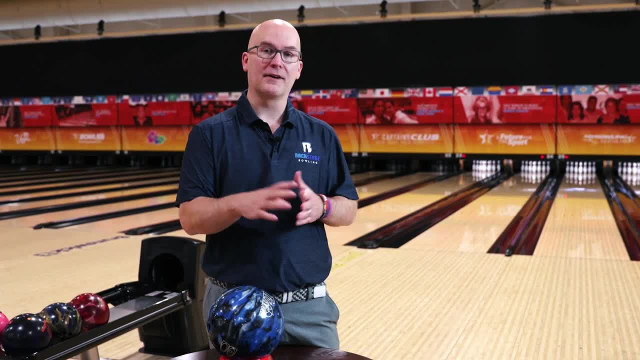 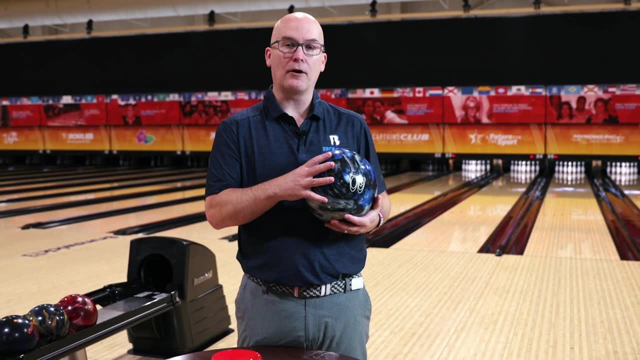 and then we can execute the shot to the best of our ability. So what are some things at home that you can sort of self-diagnose and check your span. So that's simple. So what we want to do is put our thumb all the way in to the bowling ball. 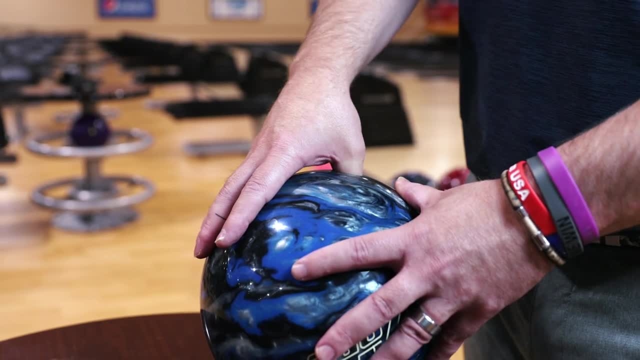 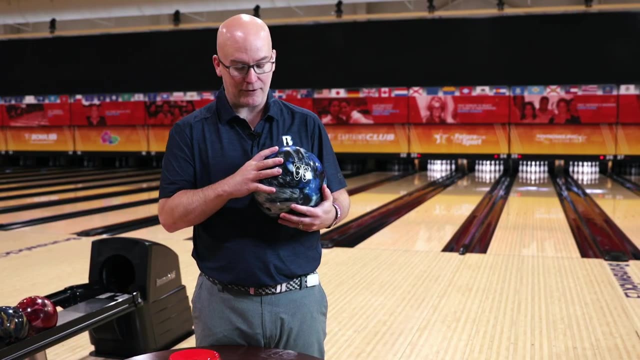 We want to make sure our thumb's all the way in and seated completely into the ball and then just lay our fingers out over the top of our finger holes. We don't want to put them inside the holes, we just want to lay them out over the top. Now, what I've done to reference here is I put a little 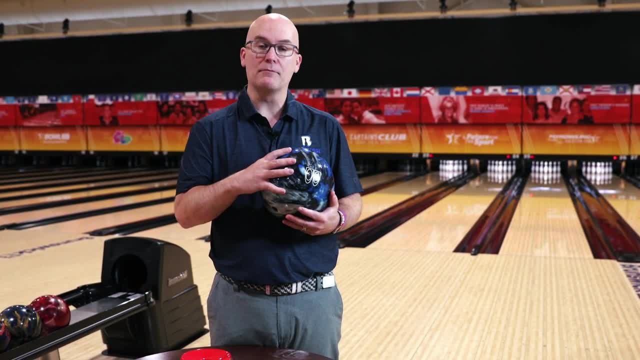 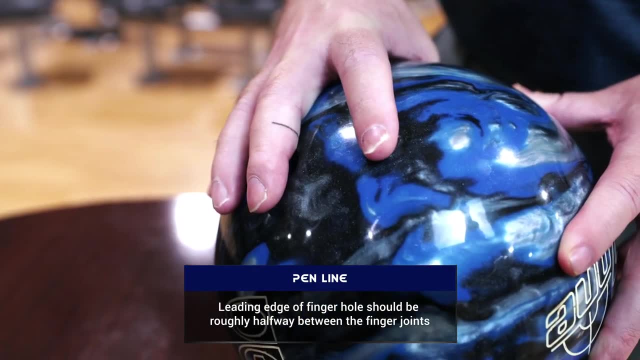 mark on the side of my fingers, directly halfway between both of my finger joints And what. we want that pen line to be lined up with the leading edge of the gripping hole. If that pen line starts to be a little bit before the leading edge of the gripping hole, we know that the spans 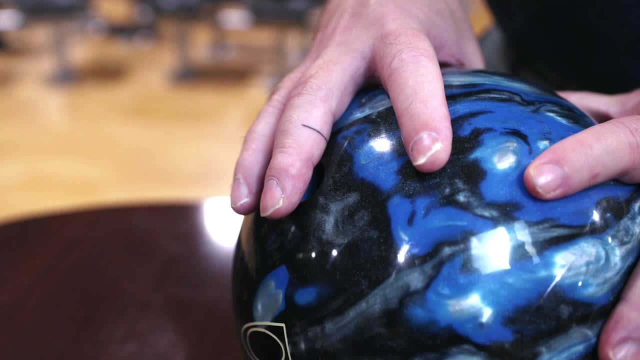 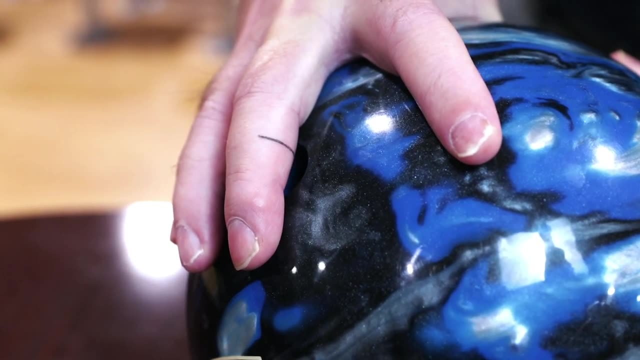 are a little bit too stretched or a little too long. Well, conversely, if that pen line ends up being more in the middle of the hole, that means our span's a little too short. Now, once again, this is just some simple at-home tips that you can do. We always are going to request you to make.